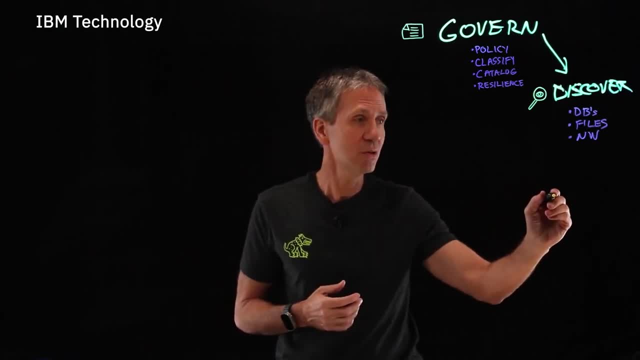 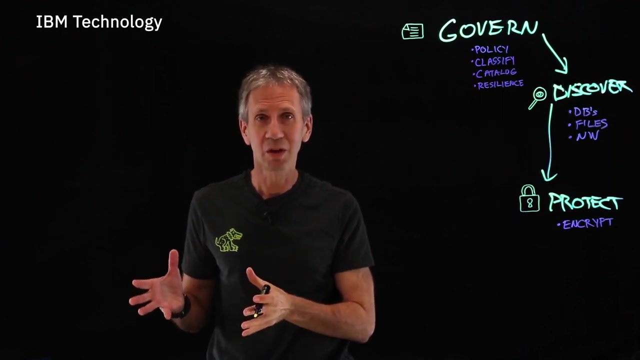 particularly important. then what's next? well then, I need to do some protection. how am I going to protect the information that I've just talked about here? I need to be able to encrypt the information so that, if it leaks out of my organization, the bad guys can't read it. I need to also have key management. if 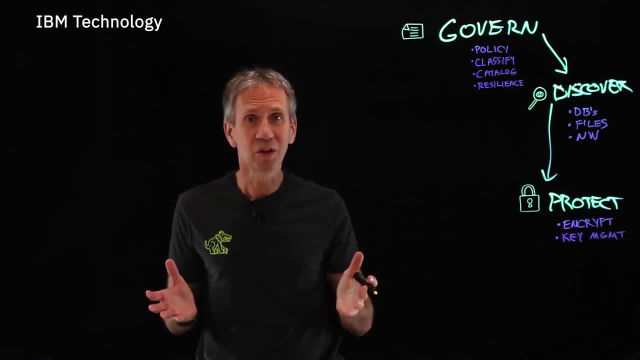 I encrypt the data and lose the keys, then I lose the data. so I have to have a key management system that generates keys securely and randomly, that stores them and keeps them secure, that tells me when I need to rotate keys and put new keys in place, so that key management system is. 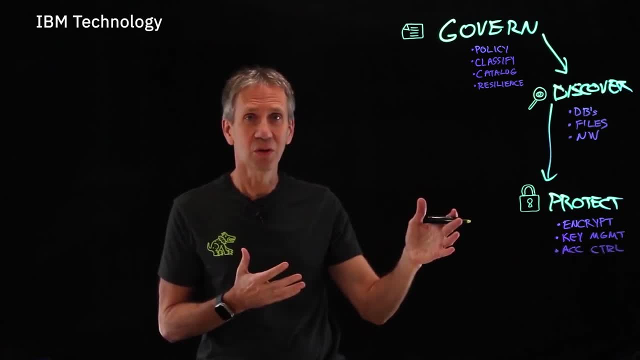 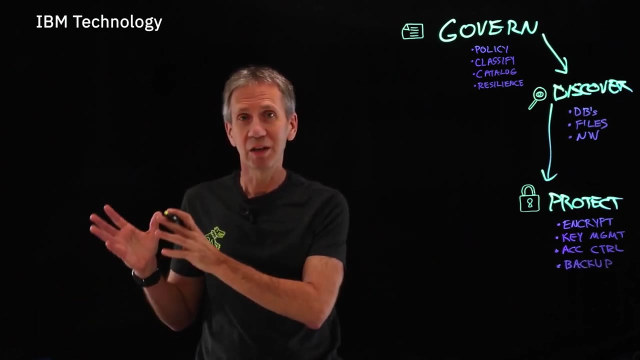 particularly important. I also need access controls: the ability to say who gets access to this and who doesn't. we could use things like multi-factor authentication, which I've talked about in other videos, and then backup, the ability to take a copy of all the data and keep it in some secure place, and 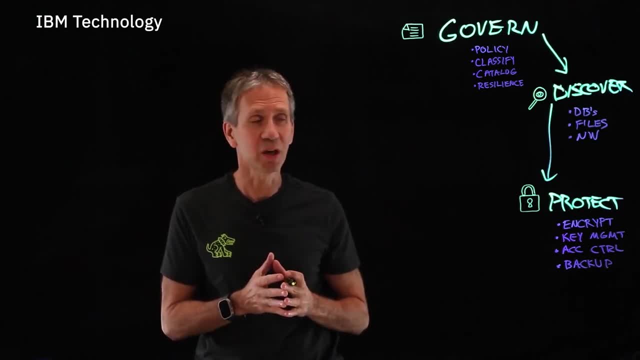 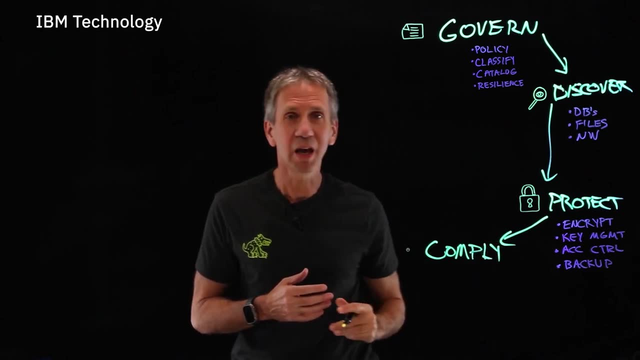 then be able to recover from that. those are the protections that I need to put in place. then, after I've done all of that, I need to ensure that I comply. we may have internal regulations that we put in place. there may be governmental regulations. there may be industry. 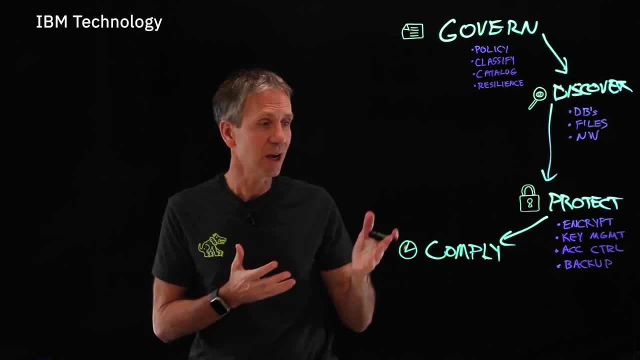 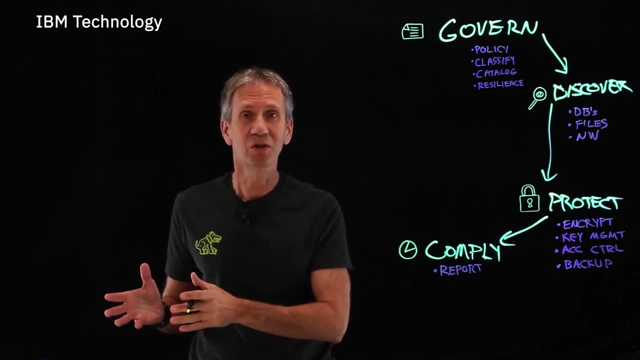 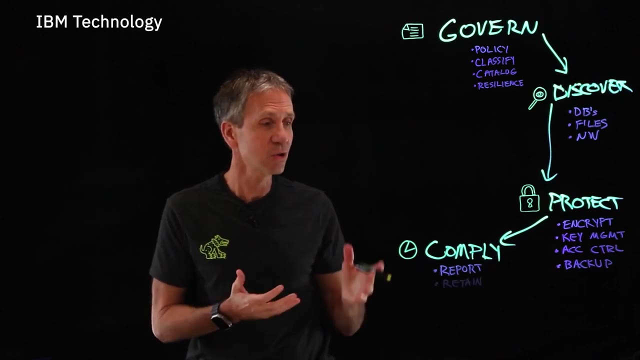 regulations that I have to follow. in some cases I need to report on those things I need to say, so the auditors will see this- that in fact I have done what I said I was going to do. that means logging a lot of information and then being able to do reporting from that. it also means retention. 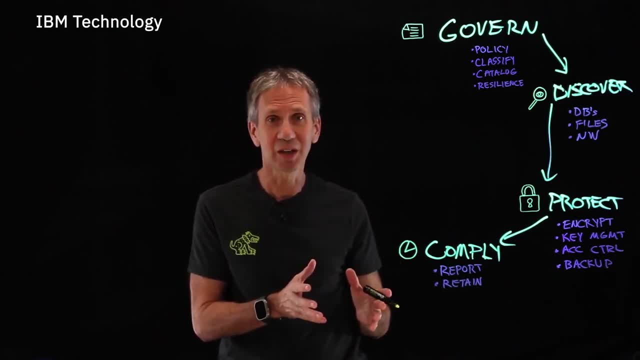 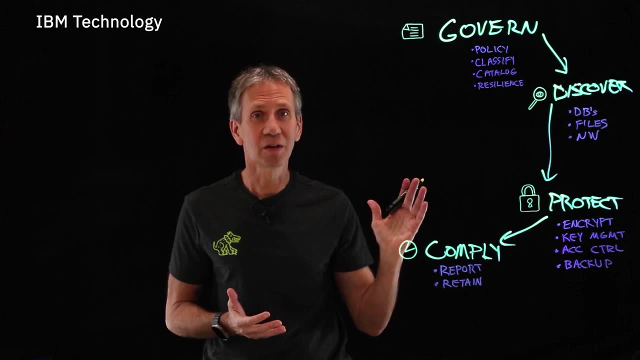 it turns out that we like to keep all the information that we ever get, but that increases our risk as an organization. it's best, once the information is no longer needed, to get rid of it. so we need a policy and an enforcement that says: this is how long I'm going to retain records, and this is 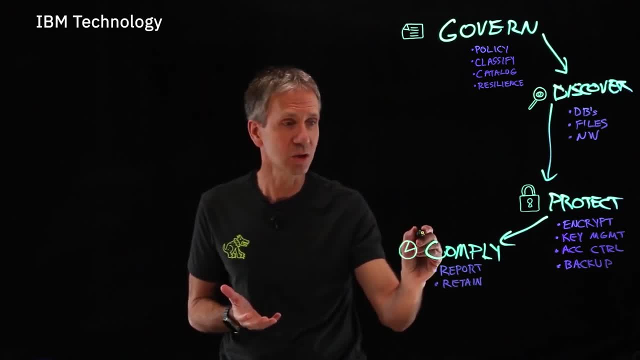 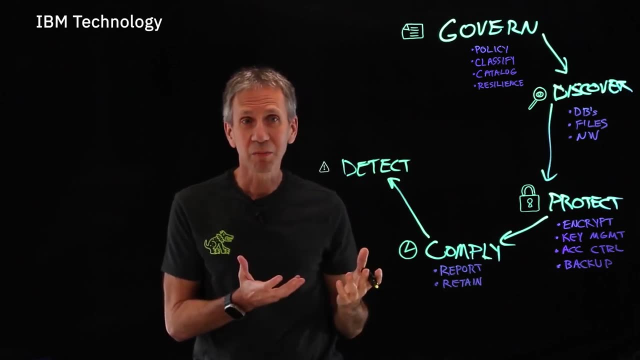 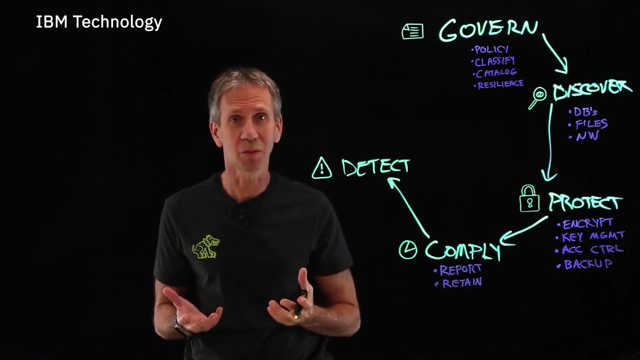 when I get rid of them so that they're no longer a risk to me and the organization, then I need ability to detect. do I have a problem? is someone using the data or misusing the data in a way that I didn't expect, in a way that is unapproved? 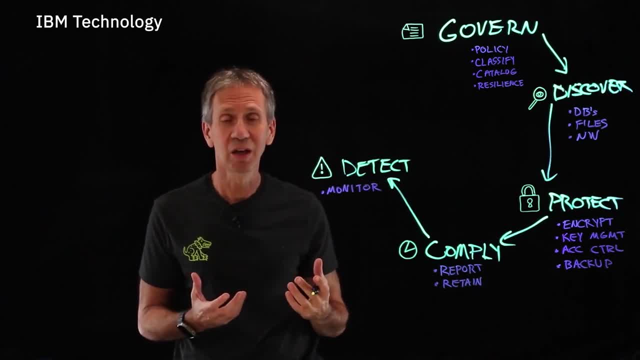 So I need a monitoring capability that lets me know that that's the case. I did a previous video on user behavior analytics, which is an example of one of those technologies That will go in and look and see when users are using data in anomalous ways. 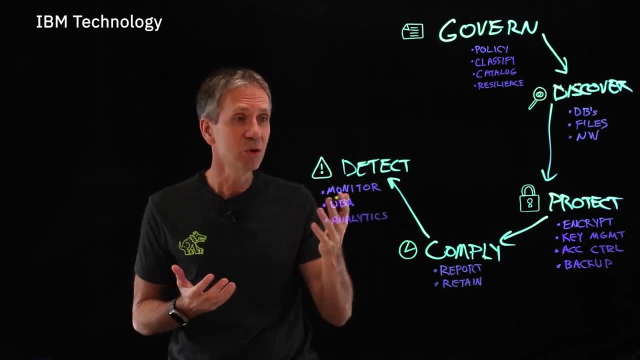 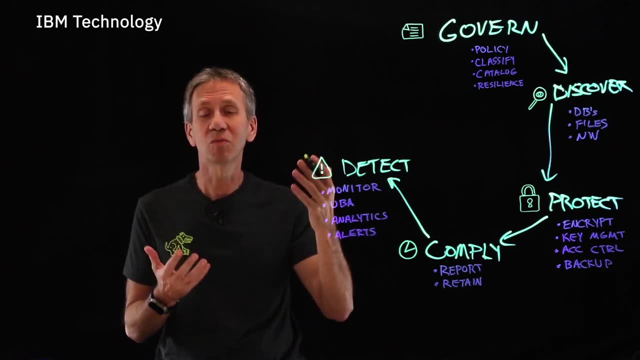 and they deviate from the norm. That would be a good trigger point. Using analytics is another way of doing this kind of analysis And then ultimately alerts that go up and tell someone we need to take action. Someone has violated or we think there's been a violation. 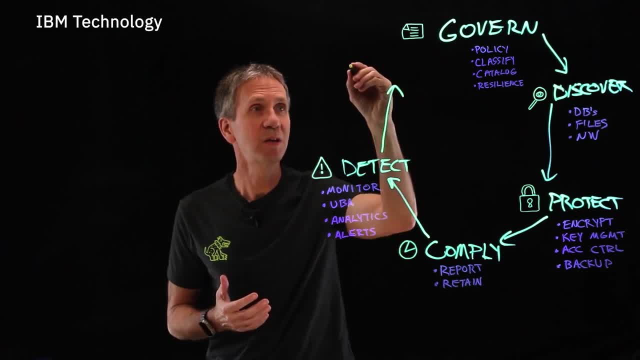 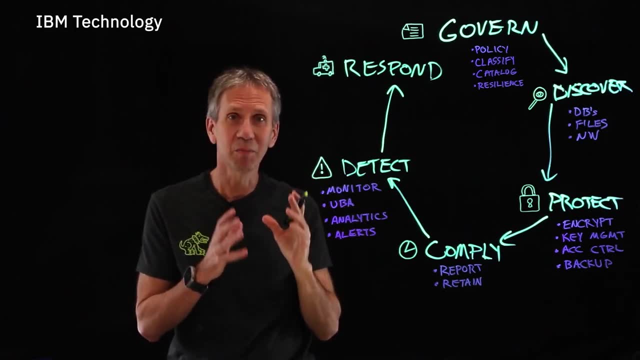 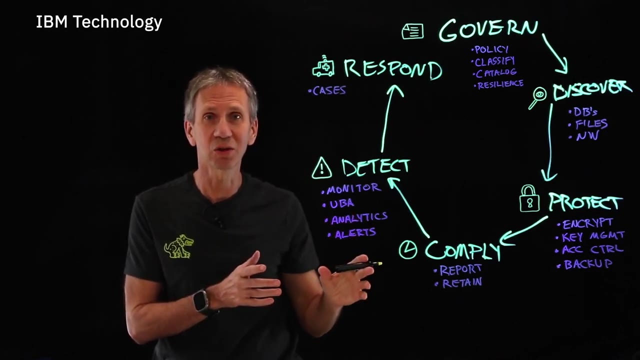 And then, once we have that, well, ultimately I need to be able to get up to a point where I can respond. When I respond, then I need an ability to create cases So with those cases I can assign those to individuals to go do investigations. 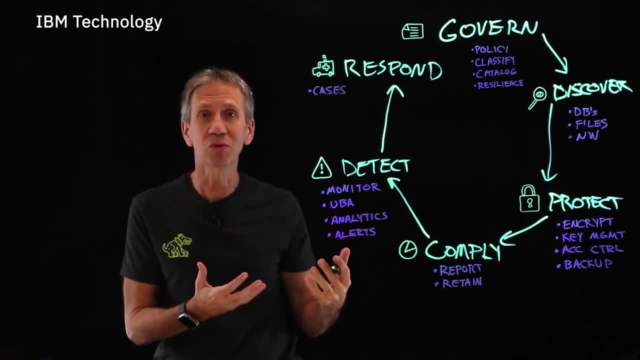 I can attach information to those. I can track them through. I can track them through to completion. Dynamic playbooks allow us to guide the analyst through what the steps should be And tell them, based upon this step, what the outcome was. 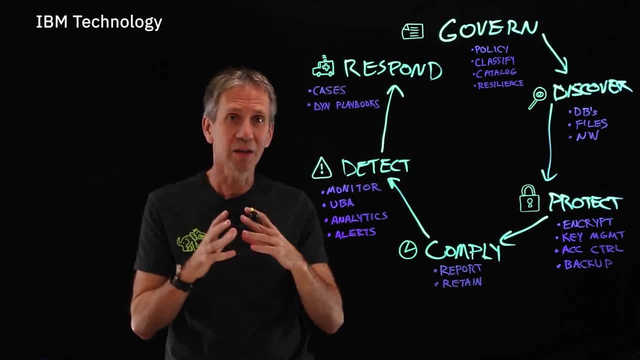 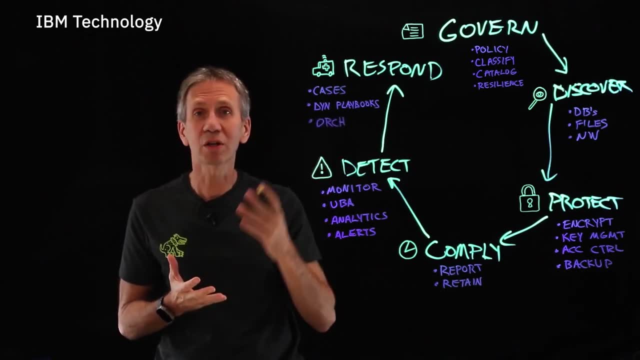 then you will do certain things to follow up against that, And it's dynamic in the sense that what you do in the second step depends on what happened as a result in the first step. We do orchestration. We'd love to automate everything, but we can't. 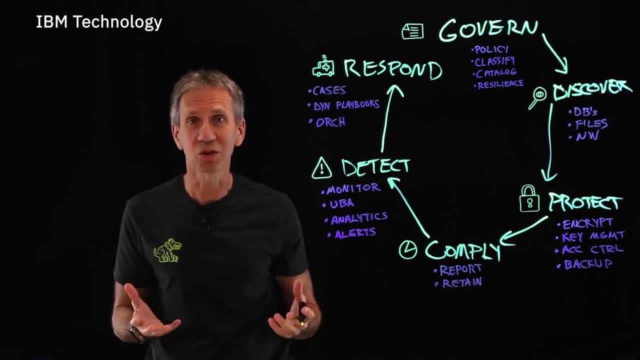 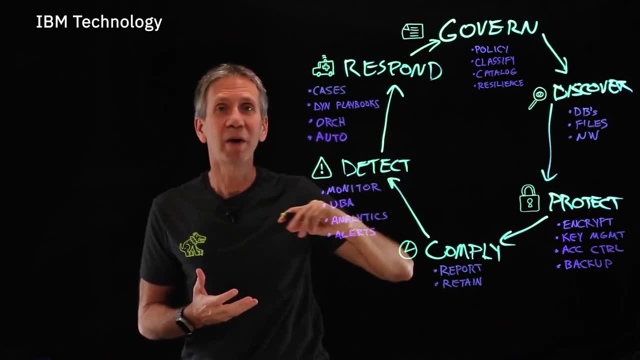 So we have to orchestrate the things that we've never seen before- the first of the kind situations, And then we automate as much as we can of the other responses. Ultimately, all of this leads back to a kind of ecosystem. Think of this as a virtuous cycle. 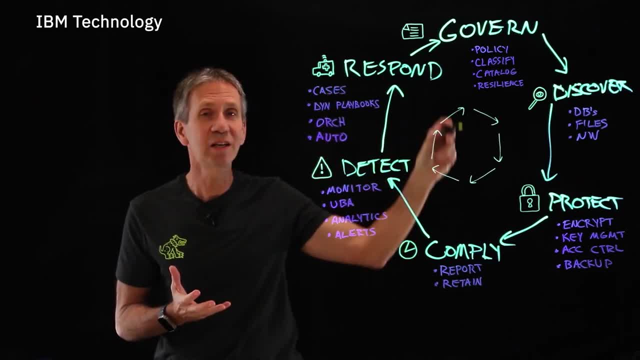 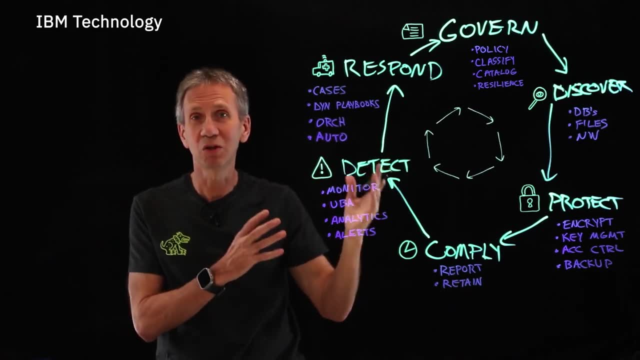 I take the information that I've learned in each of these stages and feed it into the other stages, My response tells me here's where we failed. Maybe we need to change the way we govern. Maybe we need to change our policies. Maybe that changes the way we discover information, protect it and so forth. 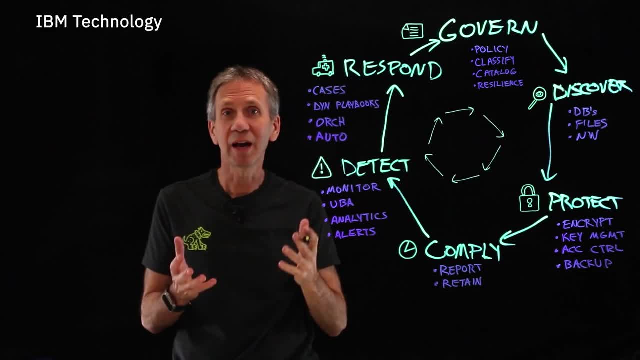 So, ultimately, what we're trying to do is create this ecosystem that allows us to protect the information that is, as I said before, the lifeblood of the organization. The good news is there is a way to do this. It requires a structured approach. 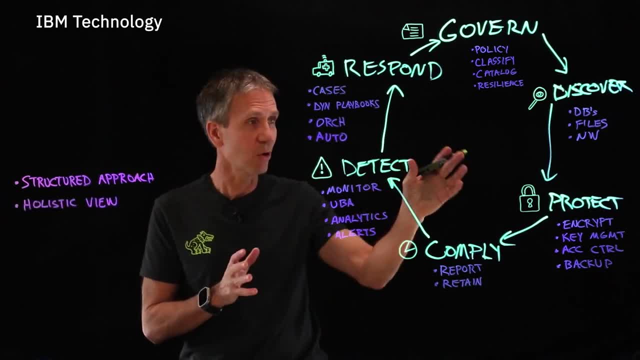 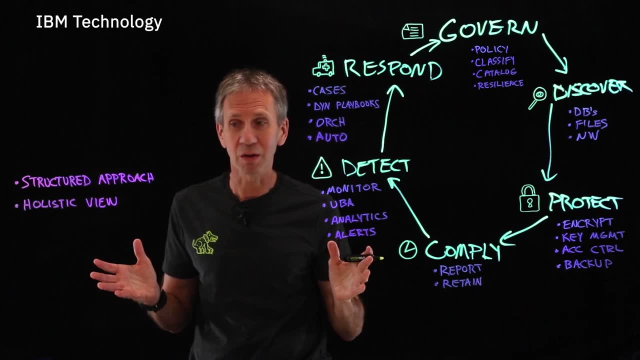 It requires a holistic view, not just looking at individual pieces, only the databases but not the files, only the structured data and ignoring the unstructured data. A holistic view is going to be critical here. Also the right architecture, Building the data security components in place, using the right. 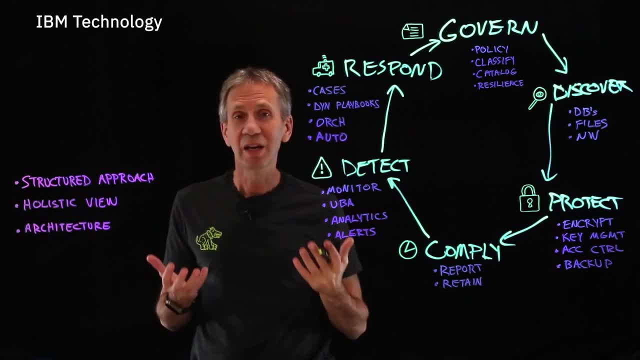 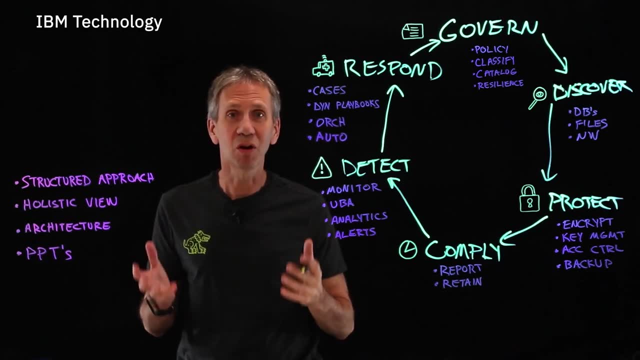 technologies- having them all integrate is going to be critical- And then, ultimately, the good PPTs, people, process and technologies. Those are the things that will ultimately implement a data security policy that makes that information available only to the people that need it, and 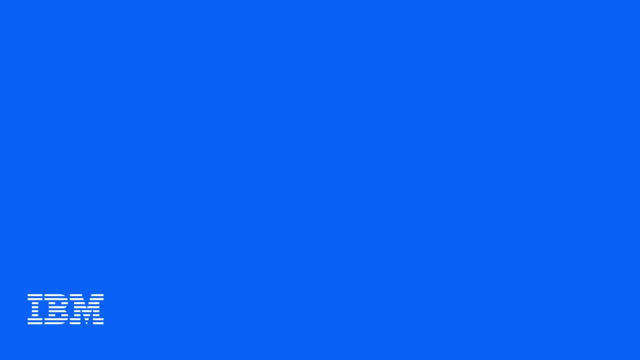 the unauthorized users don't have access. Thanks for watching. If you found this video interesting and would like to learn more about cybersecurity, please remember to hit like and subscribe to this channel. We'll see you next time. 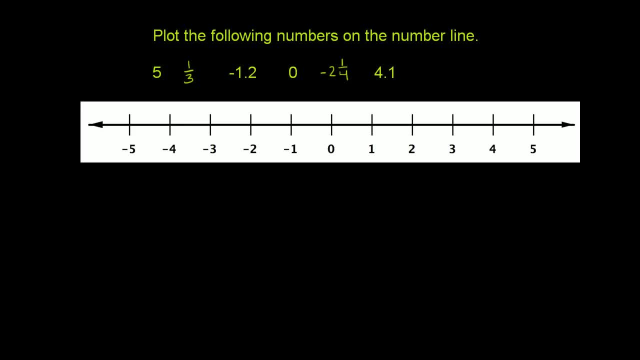 Plot the following numbers on the number line. So the first number we have here is 5.. And so 5 is 5 to the right of 0. 5 is right over there. That's our 5.. Then we get 1. third. 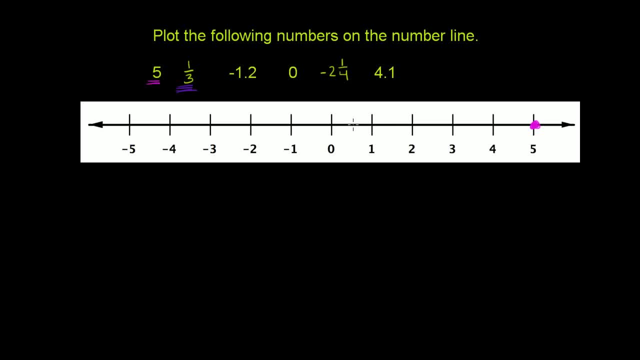 So 1 third is between 0 and 1.. And we can actually split this into thirds, So that would be 1 third, 2 thirds and then 3 thirds, which is 1.. So 1 third is going to sit right over there. 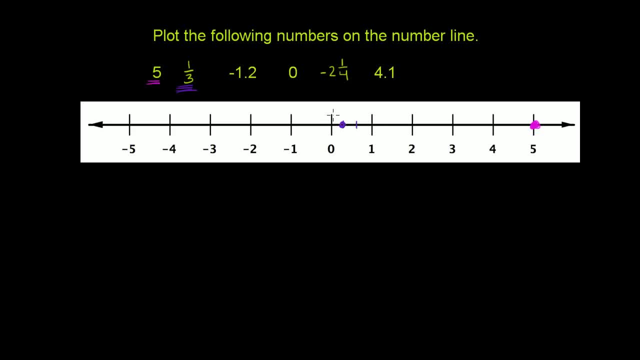 It's 1 third of the way from 0 to 1.. That's 1 third. Let me write that That's 1 third right over there. Then we have negative 1.2.. I'll do that in this blue color.